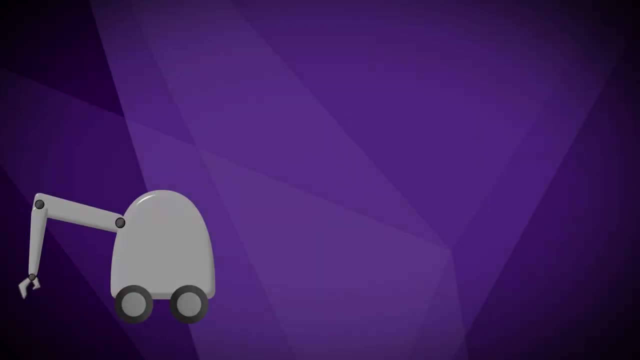 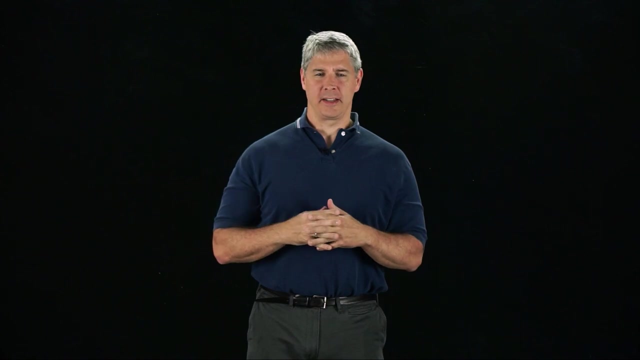 In Chapter 8, we studied the dynamics of open-chain robots. For example, the forward dynamics problem is to calculate the joint acceleration, theta double dot, given the current joint position theta, the joint velocity theta dot and the forces and torques tau applied at. 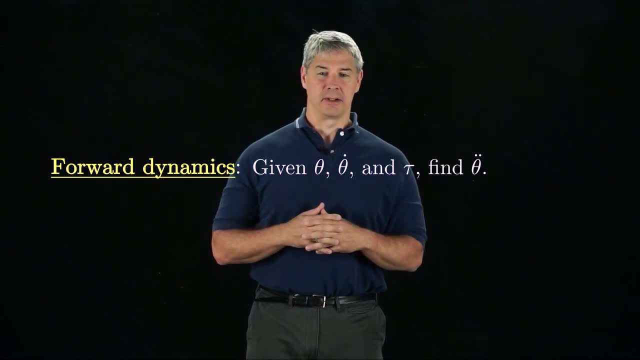 each joint. The forward dynamics is useful for simulation. The inverse dynamics problem is to find the joint forces and torques tau needed to create the acceleration theta double dot for the given joint positions and velocities. The inverse dynamics is useful in control of robots. Robot dynamics is necessary not just for simulation. 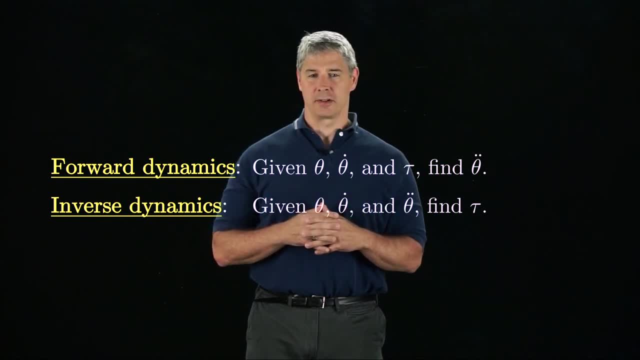 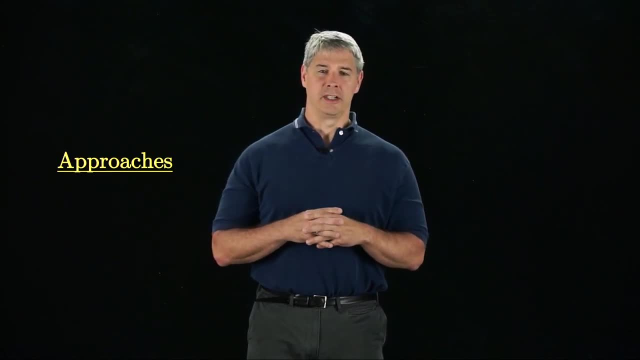 and control, but also for the analysis of robot motion planners and controllers, as we'll see in Chapters 9 through 11.. In this book we study two approaches to solving the forward and inverse dynamics problems. The first is the Lagrangian problem. 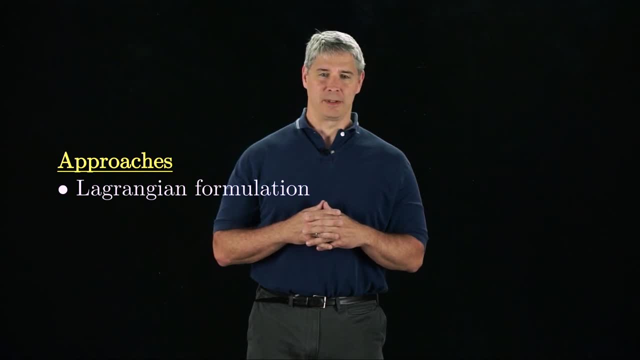 The Lagrangian formulation is a variational approach based on the kinetic and potential energy of the robot. The second approach is the Newton-Euler formulation, which relies on F equals ma, applied to each individual link of the robot. The focus of Chapter 8 is primarily on the Newton-Euler formulation because it uses: 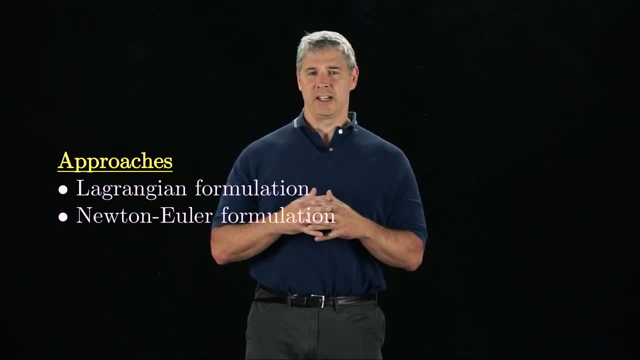 some of the geometric tools we have already developed, and it results in an efficient recursive algorithm for calculating the inverse dynamics. In this video, though, we start with the Lagrangian formulation. due to its conceptual simplicity, The key object in the Lagrangian formulation is the Lagrangian L, The Lagrangian for a. 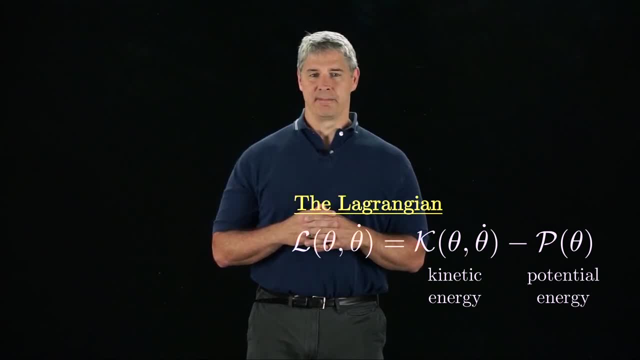 mechanical system is its kinetic energy minus its potential energy. The potential energy P depends only on the configuration, theta, while the kinetic energy K depends on theta and theta dot. I won't derive the Lagrangian equations of motion which you can find in many textbooks. 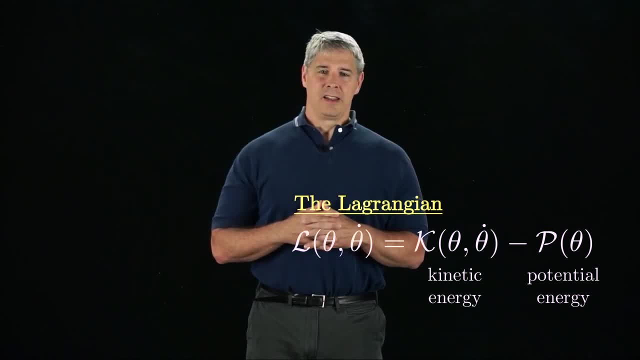 on mechanics. I'll just state the result. I'll just state the result. The vector of joint forces and torques tau is equal to the time derivative of the partial derivative of L with respect to theta, dot minus the partial derivative of L with respect to theta. 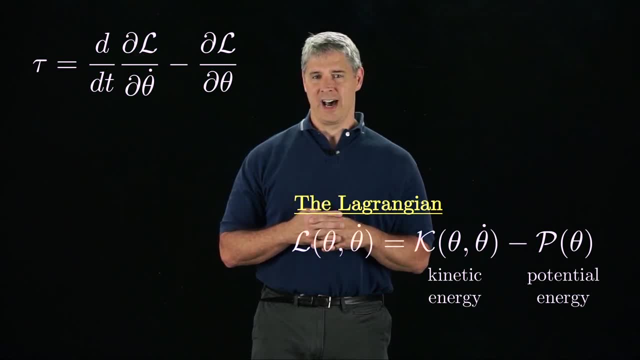 The joint forces and torques tau are dual to the joint velocities theta dot, meaning that tau dotted with theta dot represents the power consumed or produced by the joints. You can write this vector equation in its components as shown here, where tau i is the ith element of the n-vector tau. 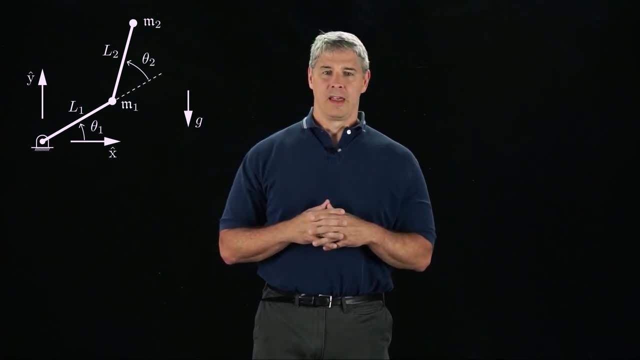 Let's apply the formulation to a 2r robot in gravity. The lengths of the links are L1 and L2 and all the mass of the robot is concentrated at point masses m1 and m2, as shown. We need to calculate the kinetic and potential energy of the two point masses. 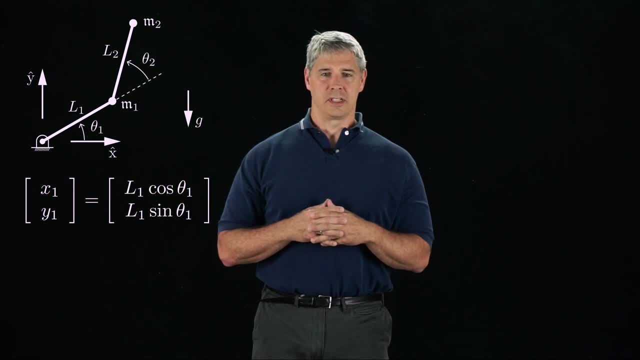 so first we calculate the position of mass 1, by the coordinates x1 and y1.. We can take the derivative to get the velocity of m1.. We can do the same for mass 2, deriving its position and velocity With this information. 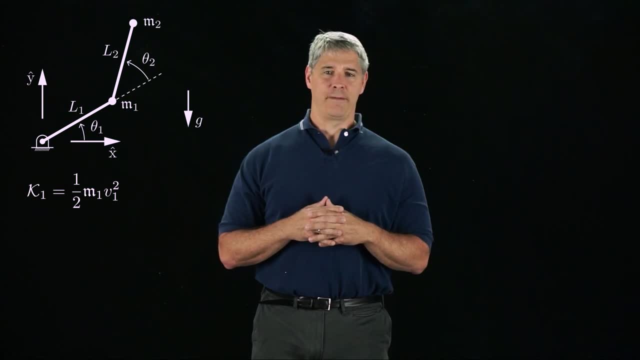 we can calculate the kinetic energy of link 1 as one-half m1 v1 squared, where v1 squared is just x1 dot squared plus y1 dot squared. Applying our earlier derivation, the kinetic energy simplifies to one-half m1 l1 squared, theta 1 dot squared. We can similarly calculate: 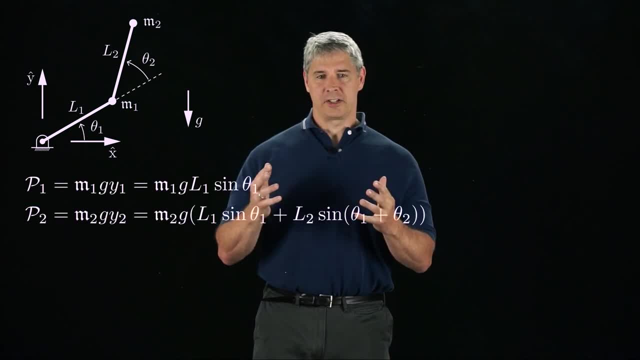 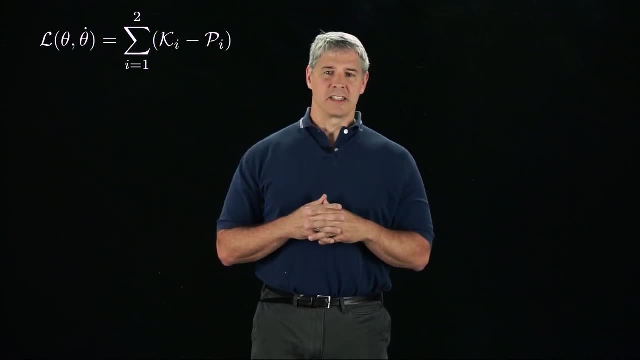 the kinetic energy of link 2.. The potential energy of each mass depends only on its height or its y coordinate. Now we can calculate the Lagrangian as the sum of the kinetic energies minus the potential energies of the links and express the joint torques in terms of. 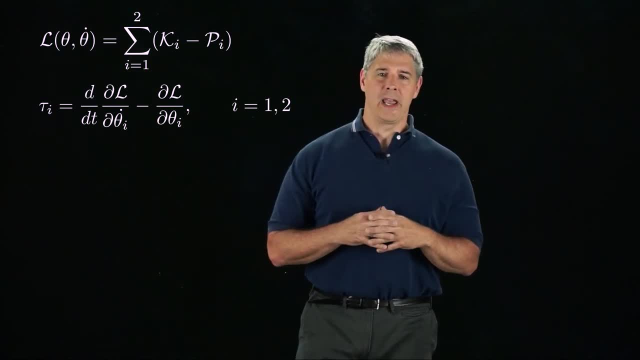 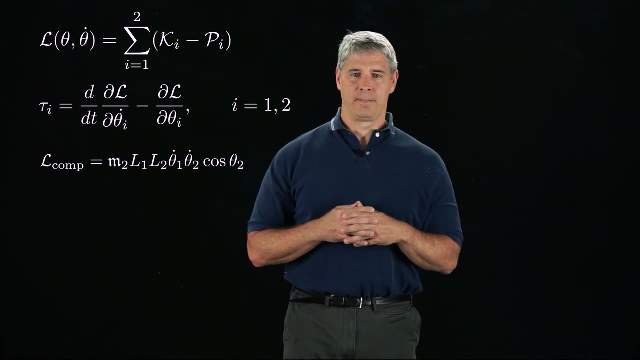 the derivatives of the Lagrangian. This is tedious to do manually, but let's look at it in a moment. Let's look at how we would calculate the derivatives for one particular component of the Lagrangian, which I'll call l-comp. The impact of this component of the Lagrangian. 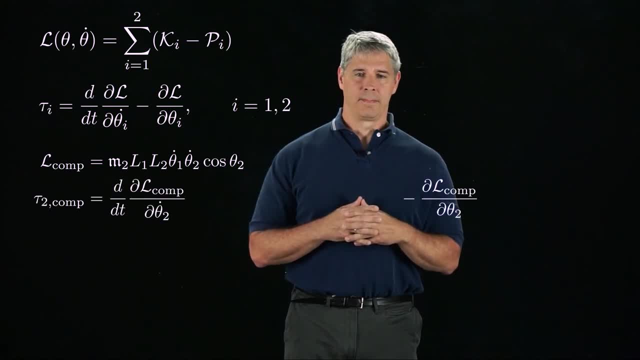 on the torque at the second joint is tau2-comp. If we take the partial derivative of l-comp with respect to theta2 dot, we get m2, l1, l2, theta1 dot, cosine of theta2.. And if we take the time derivative of that, we get the expression you see here. 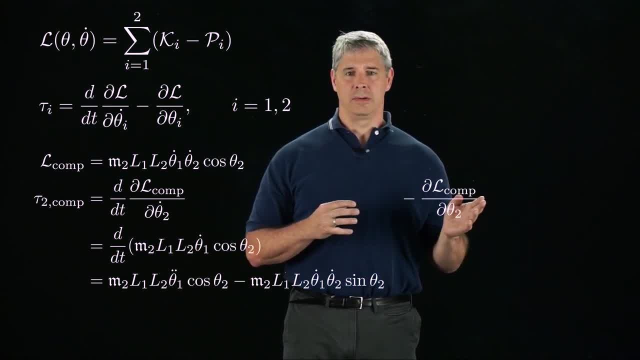 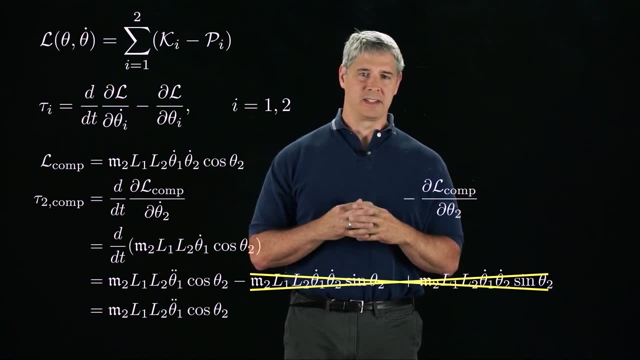 Now we can subtract the partial derivative of l-comp with respect to theta2 to get this expression. The last two terms cancel. so the final torque at joint 2 due to l-comp is m2, l1, theta1, double dot cosine theta2.. 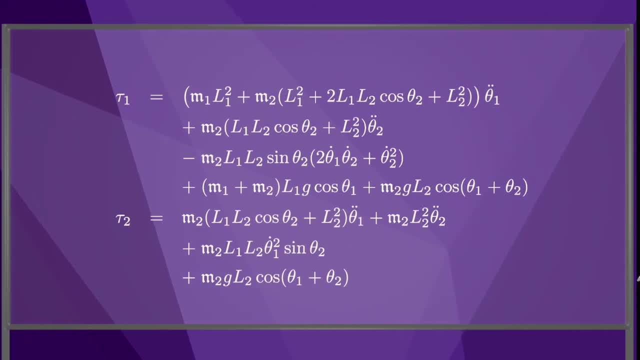 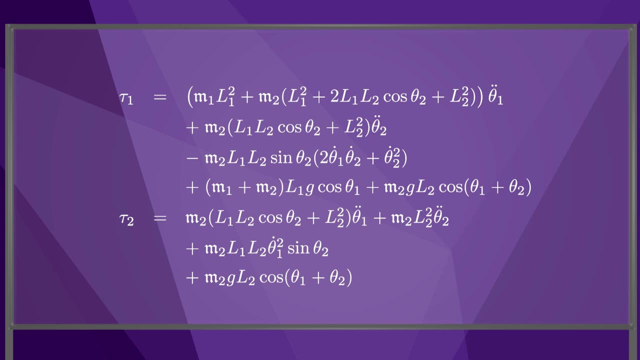 If we do these calculations for all the terms in the Lagrangian we get these equations of motion. Even for a simple 2R robot the equations are rather complicated. Notice that some terms are linear. in the joint acceleration, theta, double dot. Some terms do not have a. 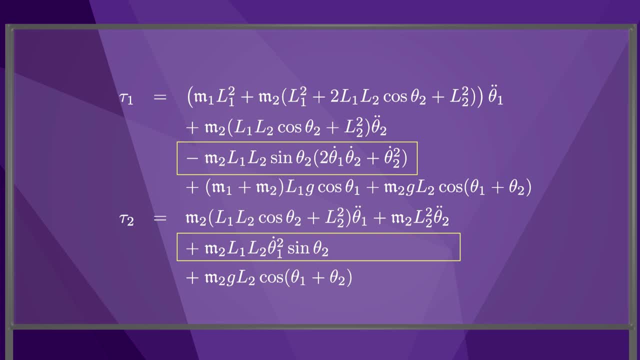 function to depend on the joint acceleration but instead depend on a product of joint velocities like theta1 dot times, theta2 dot or theta2 dot squared, And some terms have no dependence on the joint velocities or accelerations. With this observation we can write the vector. 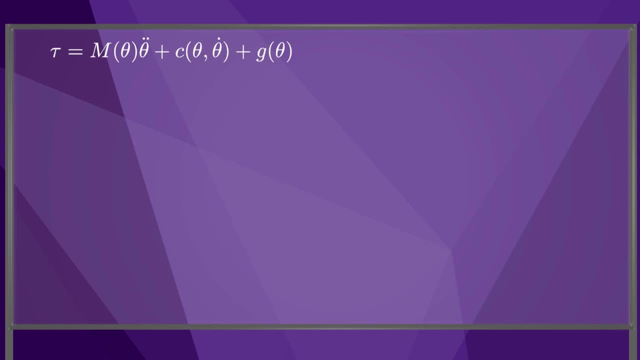 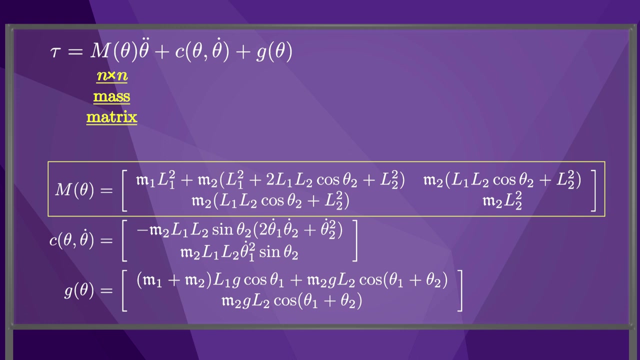 equation of motion. in this form, Tau equals m of theta times theta, double dot plus c of theta, theta dot plus g of theta, where the matrix m and the vectors c and g are shown here. What about m, the mass matrix For a robot with n joints? this matrix is n by n and for. 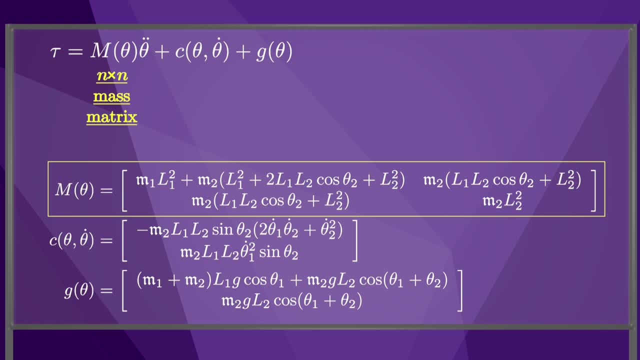 our 2R example, it is 2 by 2.. We call the vector c a velocity product term, since it is composed of terms with theta i squared or theta i times theta j in it. Finally, we call the vector g the gravity term. since it depends on gravity, We call this a gravity. 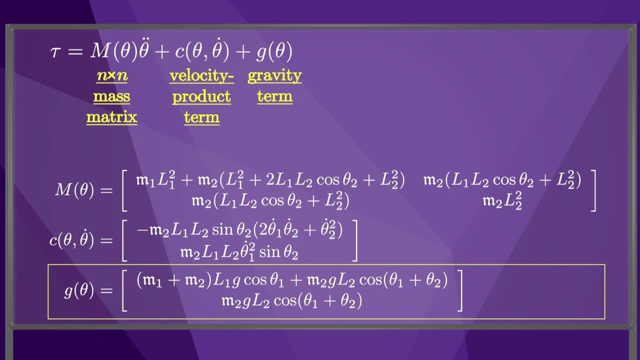 term under the assumption that the potential energy comes only from gravity. but if there were springs at the robot joints, the velocity would be greater than the potential energy that comes only from gravity. Those springs would also contribute to the potential energy and therefore to g of theta. 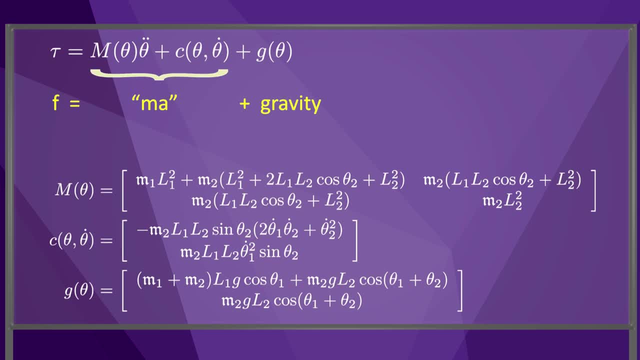 Overall, this equation looks like: F equals m, a plus a gravity force, except that the accelerations of the masses depend not only on the joint accelerations but also the products of the joint velocities. These velocity product terms appear because the joint coordinates are not inertial coordinates. We will explore velocity product terms in more detail in the